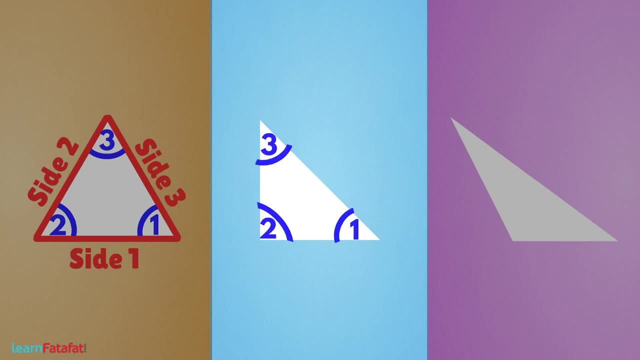 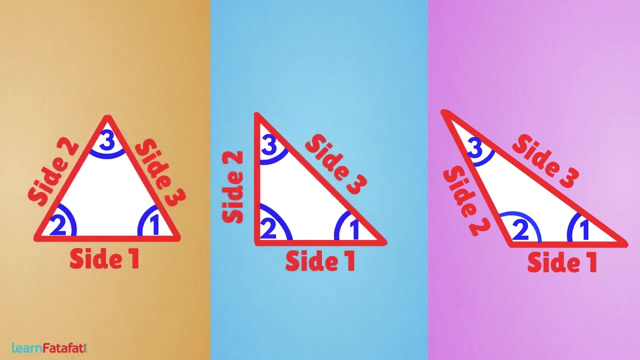 Now let's talk about this. It has 3 angles and 3 sides, So it is also called a triangle. And this: It has 3 angles and 3 sides, So it is also called a triangle. Sochni wali baat ye hai kya ye sabhi ek jaise hai. 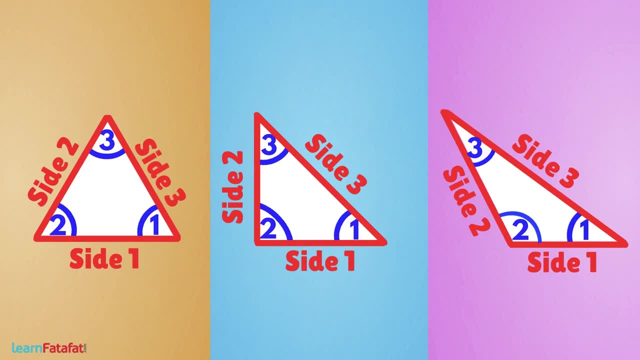 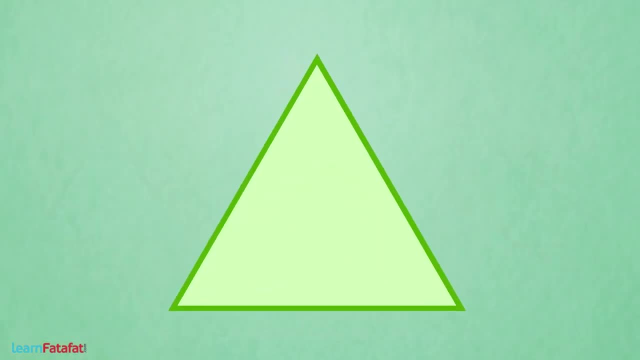 No, Ek jaise kyo nahi hai, Kyuki unke different angles hai Is triangle ki baat karte hai. Chal, ye ek L lete hai, L matlab right angle, Is angle ko hum rakhenge Triangle ke. 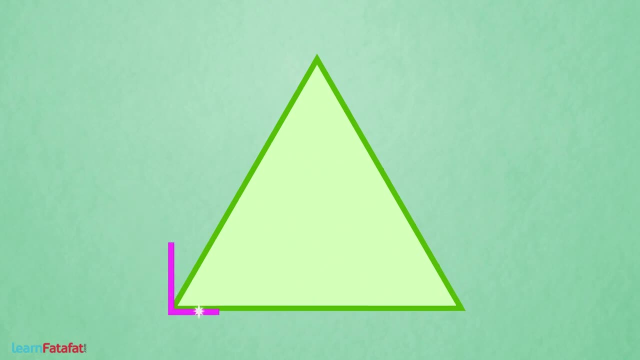 Ek angle par. Kya right angle se triangle ka angle chota hai? Haan, Agar chota hai, toh kaunsa angle hua Acute angle? Very good Aise hi, agar is triangle ke baakke angles ko bhi compare karengi. 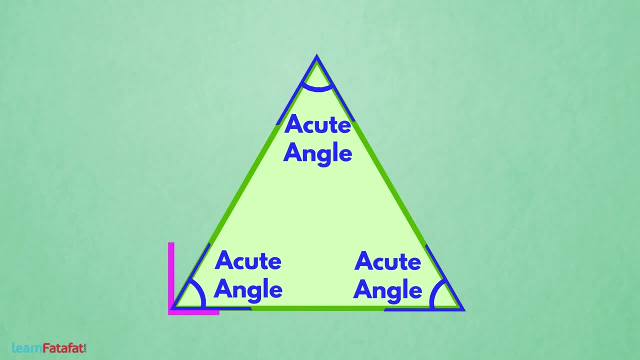 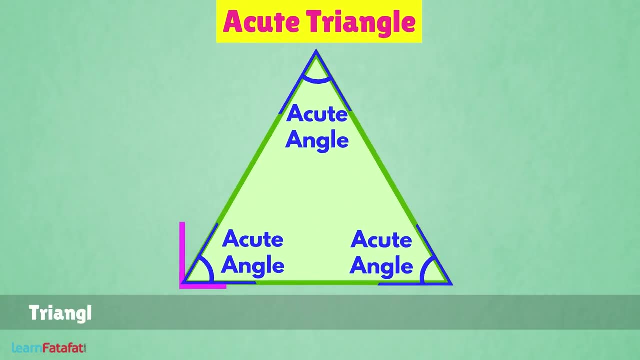 toh ve bhi chote hai. matlab acute angles hai. Aise triangle ko kete hai acute triangle. The triangle having all angles which is less than right angle is an acute triangle. Kya, ye bhi acute triangle hai. 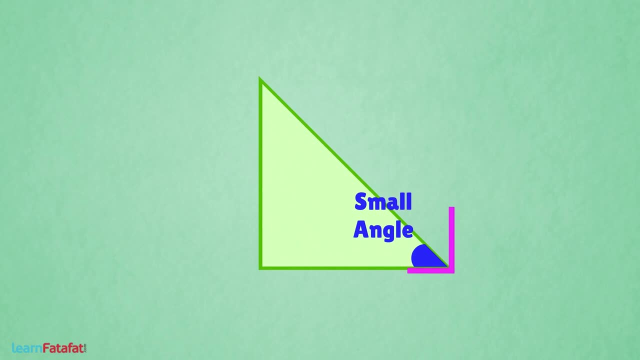 Ye angle toh right angle se chota hai. Ye bhi chota hai, lekin ye toh right angle hi hai. Aise triangle, jisme ek right angle hota hai, usse kete hai, right triangle. Ab iski baat karte hai. 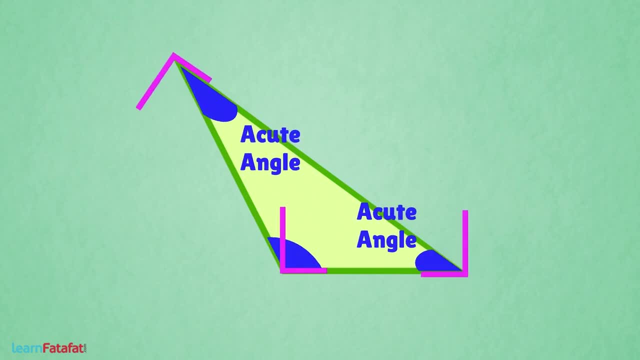 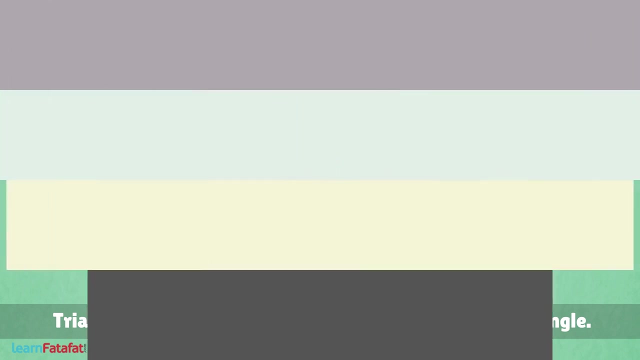 Isme bhi do acute angles hai, lekin ek obtuse matlab big angle hai. Aise triangle, ko jisme ek obtuse angle hota hai, kehlata hai obtuse triangle. Humne sikha sabhi angles agar acute hongi, toh hota hai acute triangle. 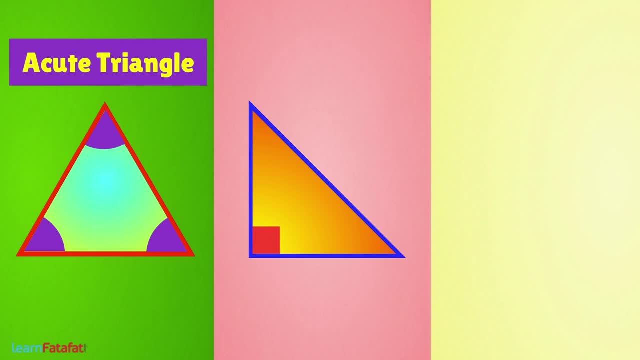 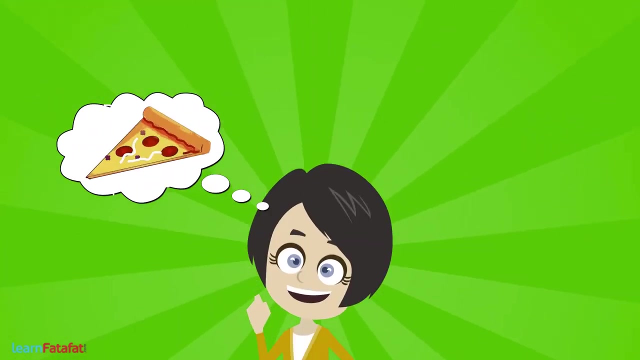 Koi ek agar right angle hota hai, toh wo hoga right triangle, Aur agar koi ek angle obtuse hoga, toh hota hai obtuse triangle. Ab sochye aapne triangle kahan dekhe hai.